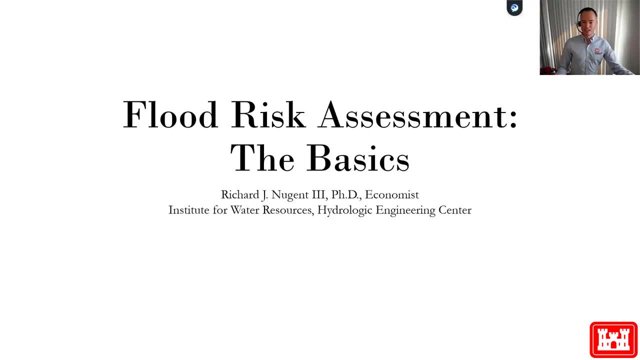 Hi all. my name is Richard Nugent. I am an economist and the lead developer for the HEC FDA program at HEC. This series of videos serves as an introduction to the topics that will be covered again and in more detail throughout the week. 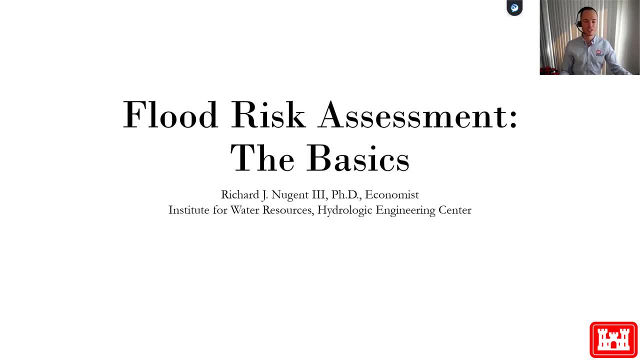 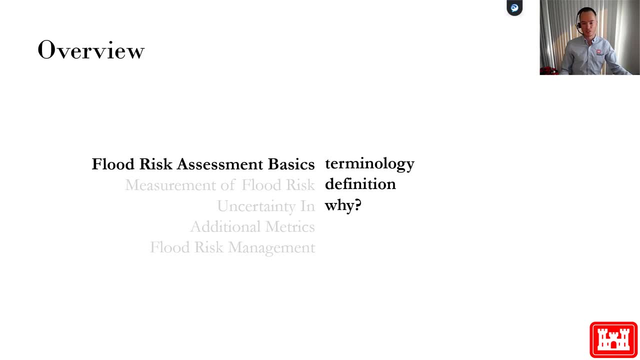 In this video we will take a look at the basics of flood risk assessment. In this flood risk assessment basics video, we will look at the terminology and disentangle a few buzzwords. We will define what flood risk assessment is and we will talk about why we measure flood risk assessment the way that we do. 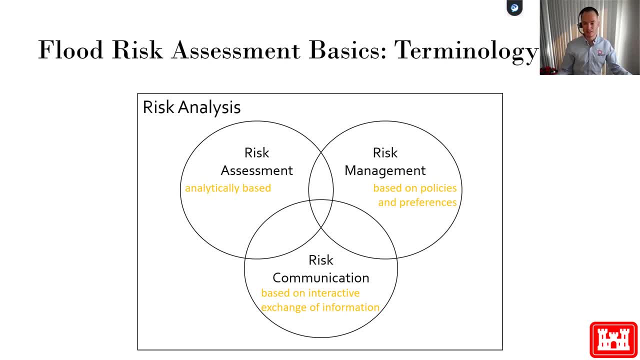 There are three pieces to risk analysis, one of which is risk assessment, The other two are risk management and risk communication. Each of these pieces of risk analysis represents an important and independent, but also related- concept, as illustrated by the Venn diagram. Risk assessment is analytically based and involves measuring and quantifying risk through science and analysis. 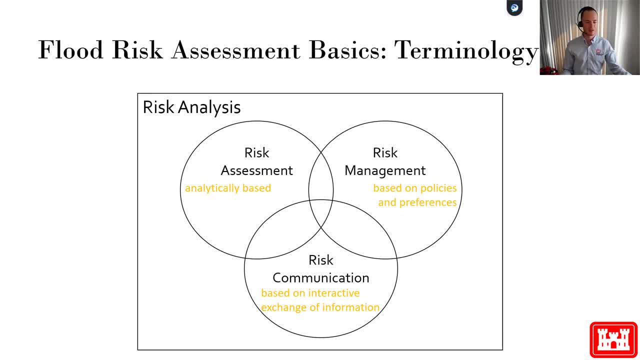 Risk analysis is the work in which most economists and engineers at the core are involved. Risk management deals with the reduction or mitigation of the assessed risk. Risk management is driven by policy preference and leadership decisions. For instance, we could drive flood risk close to zero by moving us all up atop a mountain. 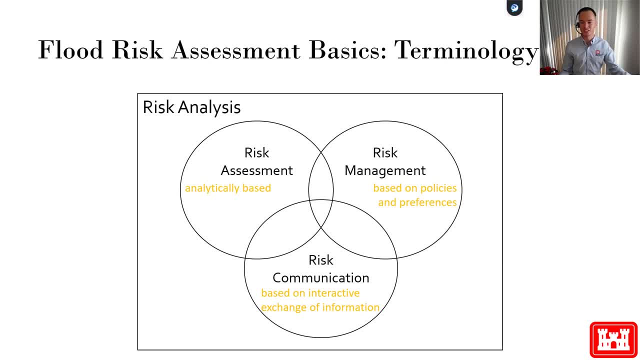